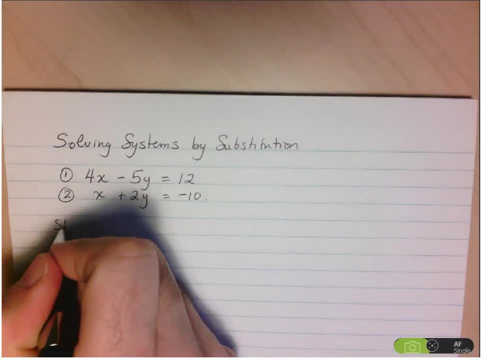 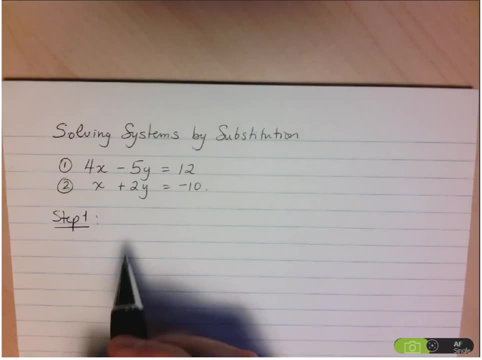 we won't end up with any fractions. So step 1 for solving systems by substitution is to choose a variable to isolate. Now, of course, you could use it even if they all had coefficients, but it would make the process a little more difficult. 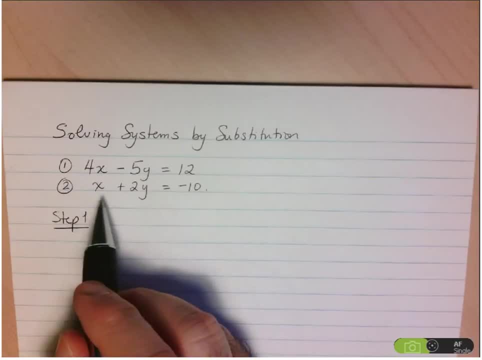 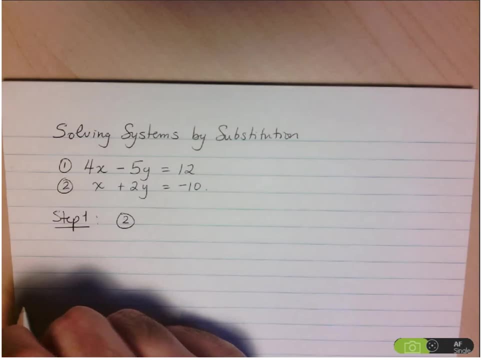 So step 1: here, clearly, equation 2 is the one to pick, because the x variable has a coefficient of 1.. So the first thing I'm going to do is take equation 2, and I'm going to isolate x, So x here and I just take the 2y to the other side. 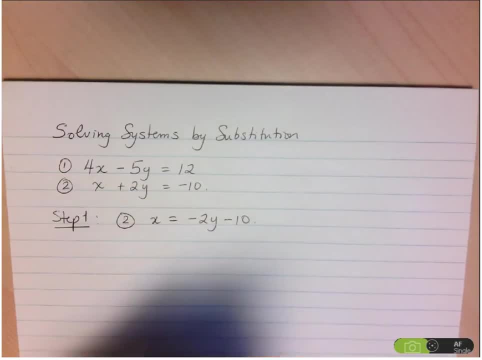 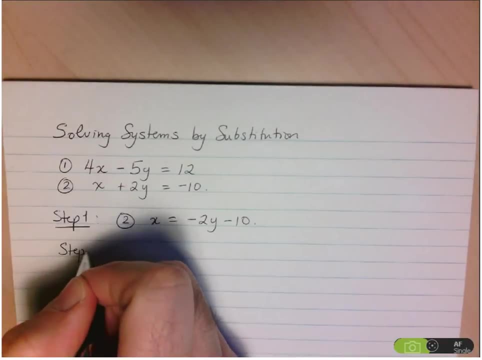 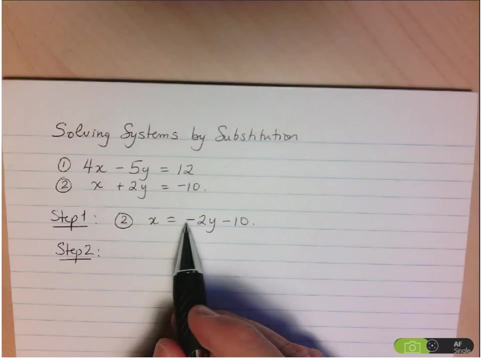 and I end up with negative 2y minus 10.. And that's it. Just find the variable and isolate it. Step 2, and this is where the title of the method comes into play- is we substitute this expression in the other equation. 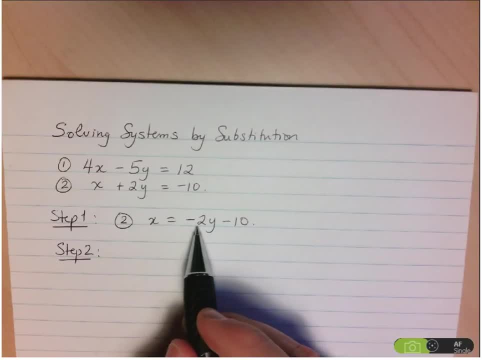 where we see x. So x is equal to 2y minus 10.. Hence, anywhere I see an x, I can just now replace it with what it's equal to, which is negative: 2y minus 10.. So we always substitute into the equation we haven't used. 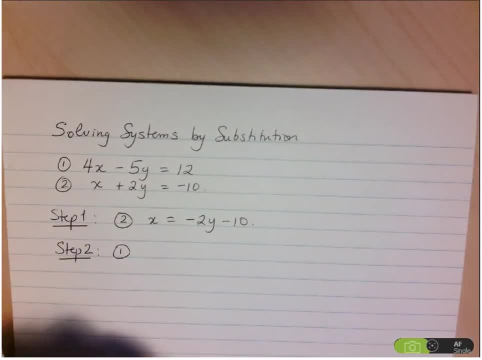 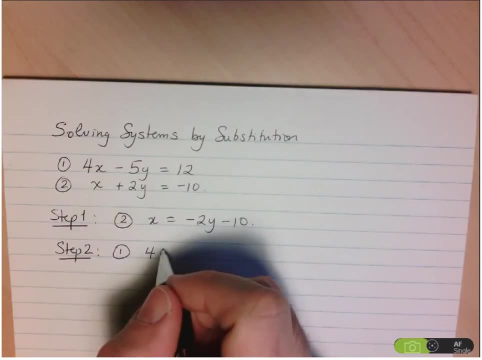 So that's why here I have to use equation 1.. So equation 1 is: 4x minus 5y, equals 12, whereas I'm going to now substitute x for its equivalent expression, which is negative, 2y minus 10.. 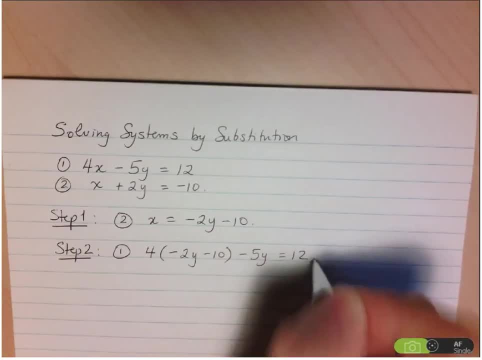 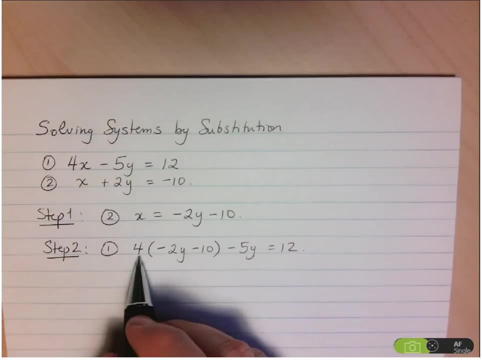 Then I've got minus 5y equals 12.. Now what I have is one equation with one unknown, and this is something I can solve. So we start by distributing the 4. So we have 4 times negative 2y. 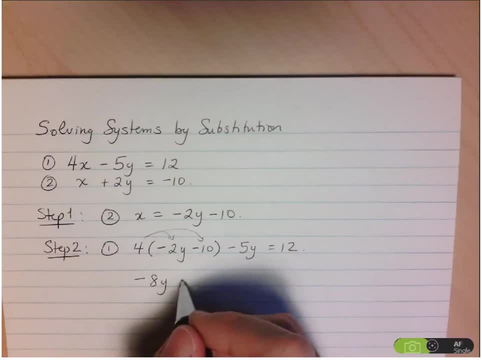 negative 8y, and then 4 times negative 10 minus 40, and minus 5y equals 12.. Bring the y's together, so negative 8 minus 5, we have negative 13y, And then here we have 12 plus 40,. 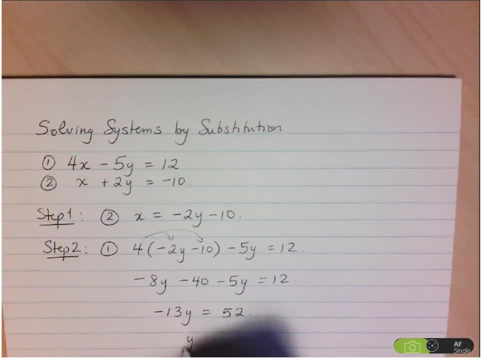 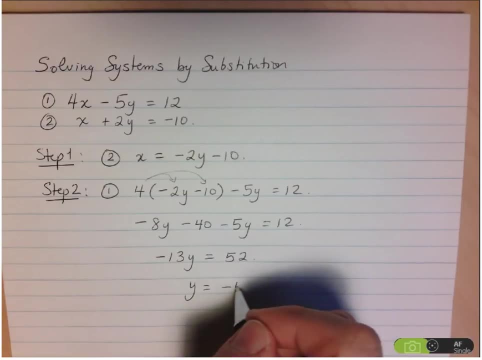 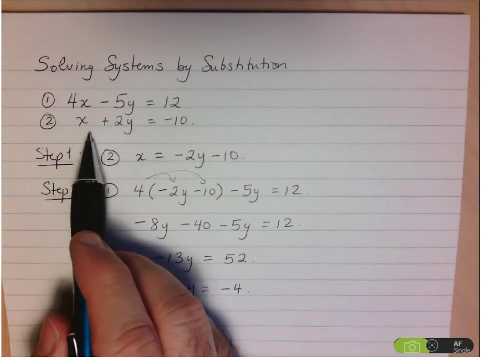 so that's just going to be 52. And then to solve for y, we just divide 52 by negative 13, and that's negative. So now we've found the y value. that will help to solve this system of equations. But there are two variables.